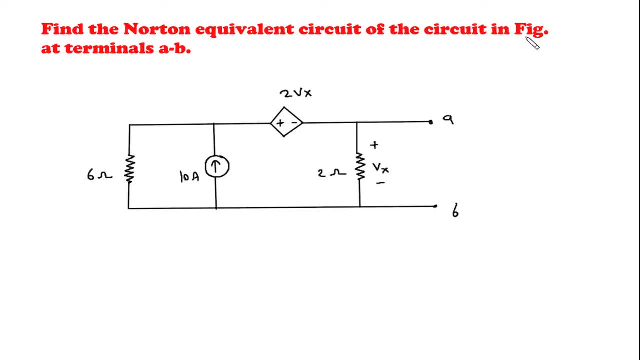 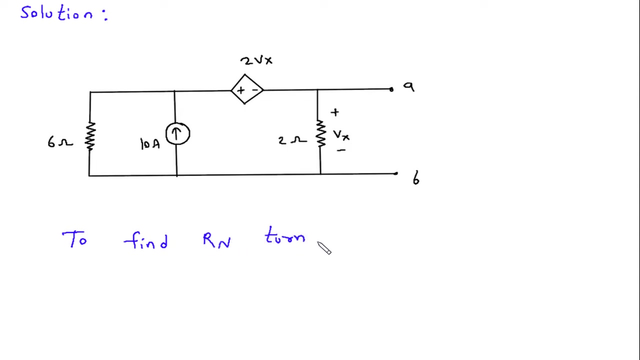 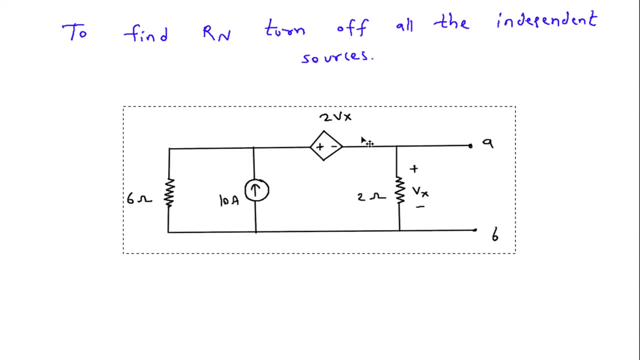 Find the Norton-equivalent circuit of the circuit in figure at terminals A, B. Solution. First we will redraw the circuit. Now we will find To find Rn- Turn off all the independent sources. So we will turn off all the independent sources. 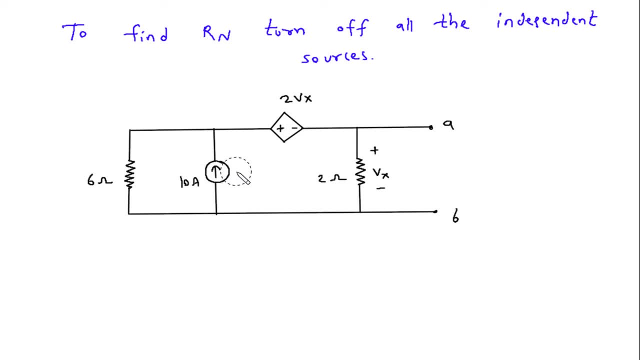 This 10A is the current source, So this will be Turn off. When we turn off the current source, then that will be an open circuit. Now this 2Vx is the dependent source, So To find Rn we will apply 1V. 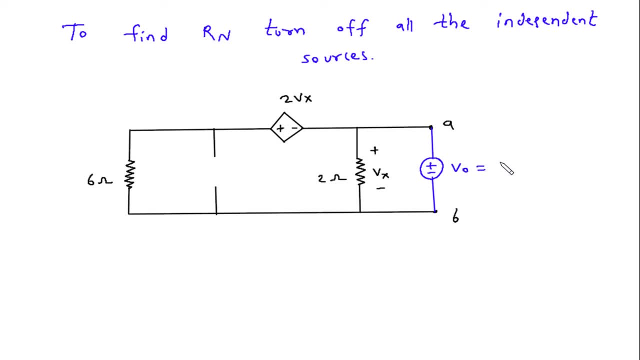 voltage source. Let's say this is Vo with 1V and this is Io. So from this we can find the value of Rn. Rn will be equal to Vo, which is 1 by Io. So we need to find Io to find Rn. 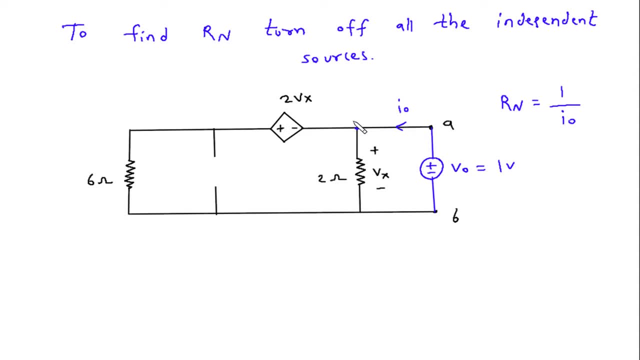 So to find Io, Let's say this is node Va, This is grounded. Now let's say this is current I1.. Let's assume This is I1.. This is I2.. So apply KCl at node Va. So summation of all. 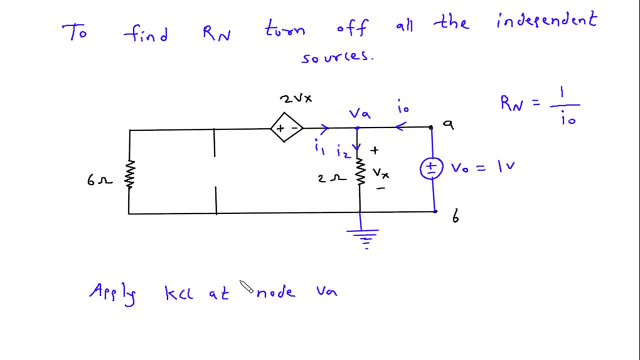 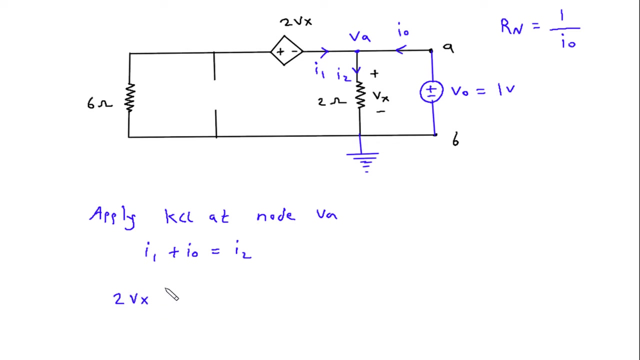 the entering current. Entering current is I1 plus Io. I1 plus Io is equal to I2.. I1 will be This: will be 2Vx minus 2Vx minus Va, minus 2Vx minus Va by 6, then plus. 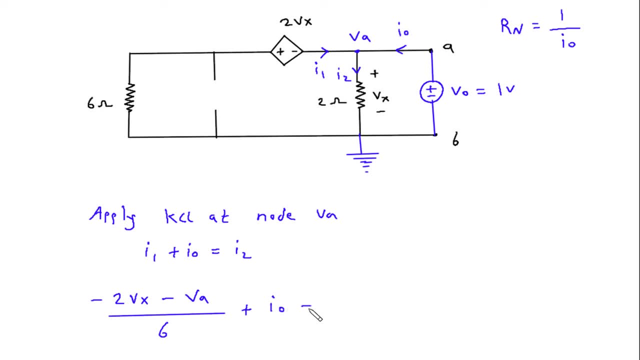 Io then is equal to I2.. Now I2 is Va minus 0, Va minus 0 by 2. Now, as we can see that Vx is connected to ground, This Va is also connected to ground and across Va and Vx, this Vo is. 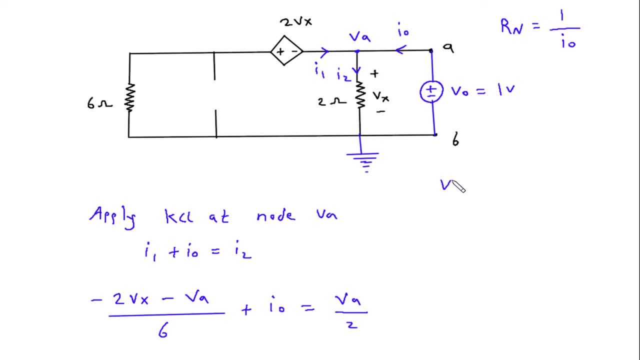 connected. So Va and Vx is equal to 1. Va is equal to Vx is equal to Vo is equal to 1. 1V. So from this this will be: Io is equal to Va by 2. or directly 1 by 2, then this will be: 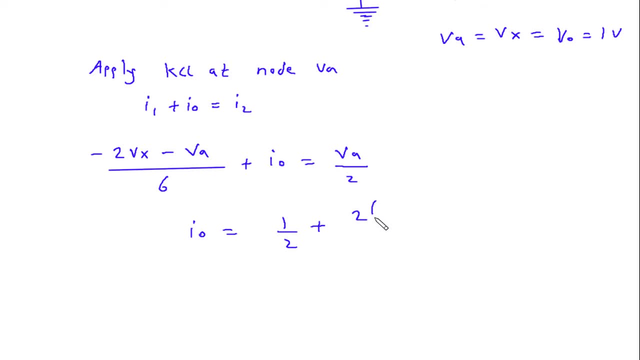 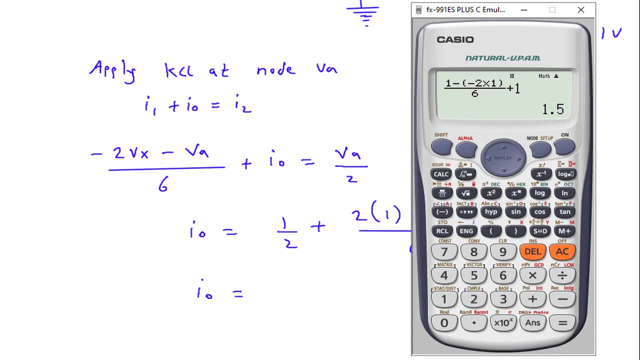 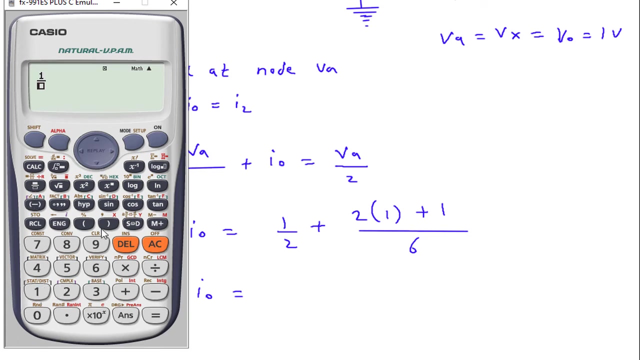 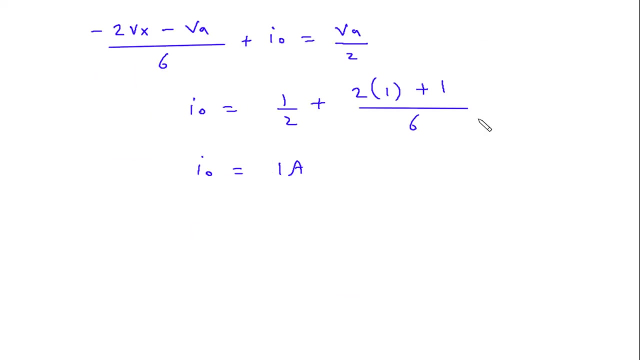 plus 2 into 1, then plus this will be 1 by 6.. So Io is equal to 1 by 2, then plus 2 into 1 plus 1 by 6, So this is equal to 1. Ampere Rn is equal to. 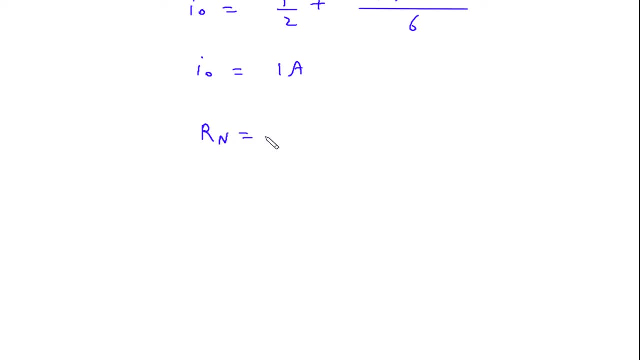 1 by Io, Rn is equal to 1 by Io. So 1 by 1 is equal to 1 Ohm. Therefore, Rn is equal to 1 Ohm. Next we have to find. I In, I So to find, To find. 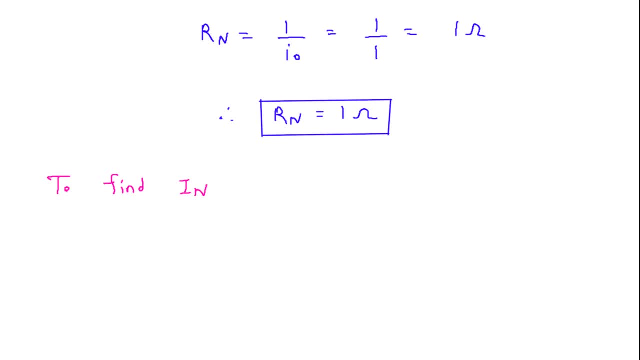 To find I in short circuit terminal terminal AB short circuit. So this will be short circuited and this will be current IN Now when we short circuit A and B Vx is equal to zero. this Vx is equal to zero, so this: